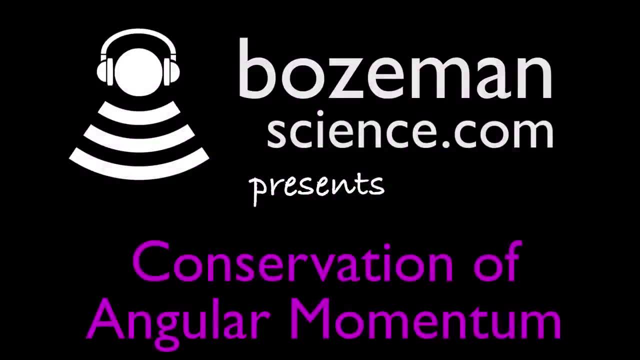 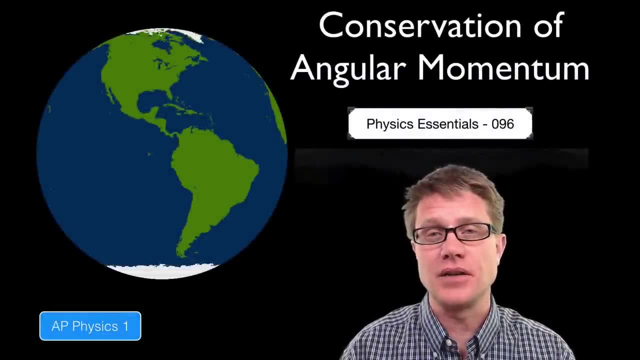 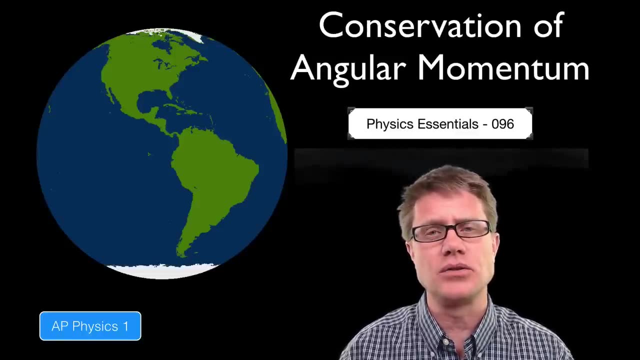 Hi, It's Mr Andersen and this is AP Physics essentials, video 96.. It is on the conservation of angular momentum. Now, how is angular momentum different from linear momentum? Remember angular momentum is due to rotation, And you might think to yourself. 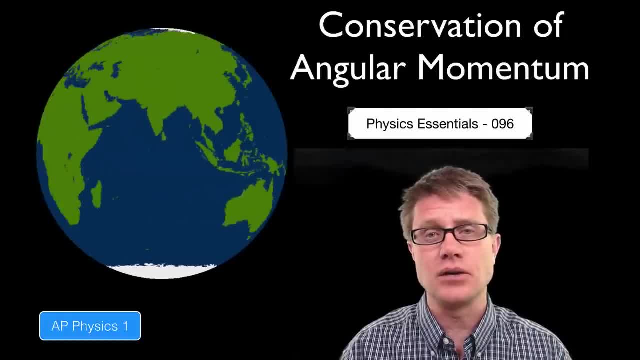 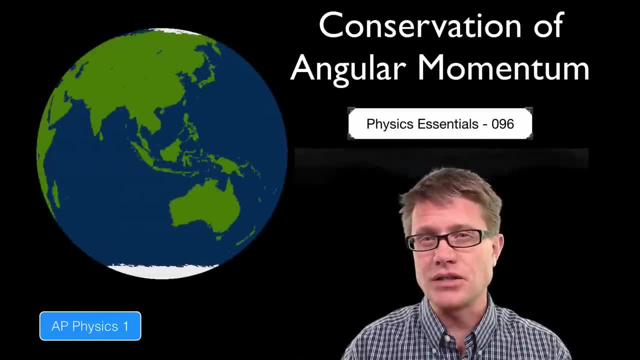 why does the earth continue to rotate? It is due to the conservation of angular momentum. It still maintains some of that angular momentum from the formation of the solar system. It is gradually slowing down and it will eventually stop, But it is not something that we have. 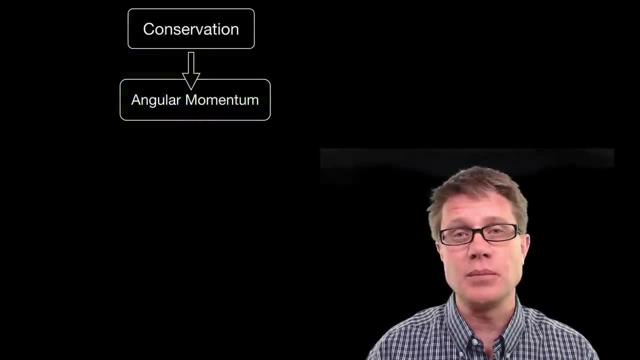 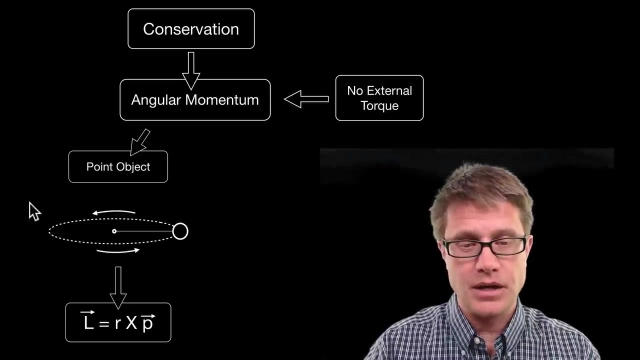 to worry about. So conservation of angular momentum will always be maintained as long as we have no net external torque acting on an object or acting on the system itself. Now, unlike linear momentum, we can calculate angular momentum in one of two ways. If it is a point object in rotation, then our angular momentum is equal to the radius of the angular 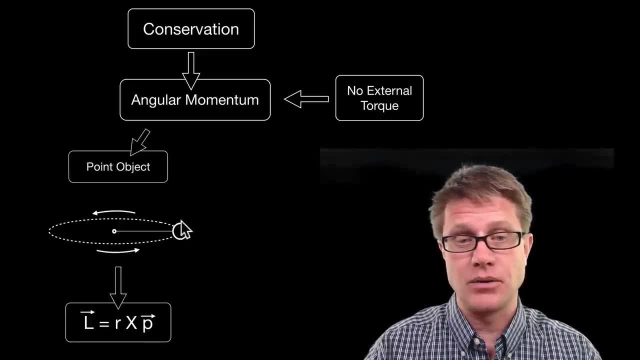 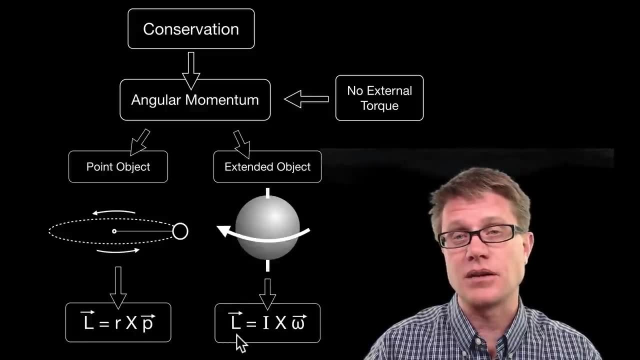 momentum times the linear momentum of the object. So how fast it is going in this direction times its mass. If we have an extended object, we use a different equation. If we are an extended object, the angular momentum is equal to the moment of inertia. so that is how much. 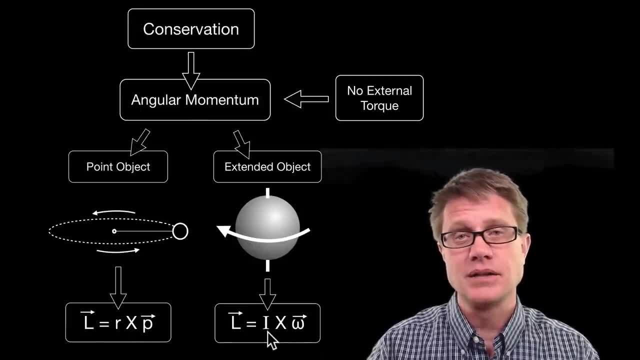 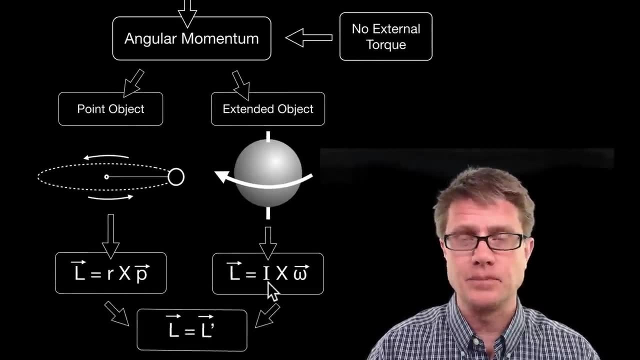 material we have and how far it is spread out from the center times the angular velocity of the object. But in both cases, as long as there is no net external torque acting on it, the angular momentum before equals the angular momentum we have after. Now I 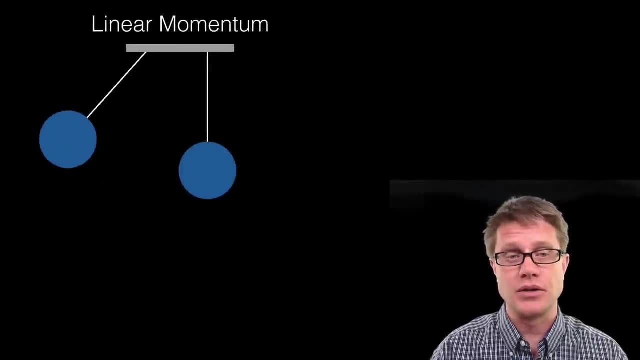 again, there are analogs for linear momentum. Remember, in linear momentum, during a collision like this, the momentum is simply transferred between the two. Now, in linear momentum, linear momentum equals mass times, the velocity of the object. But we have analogs when we are. 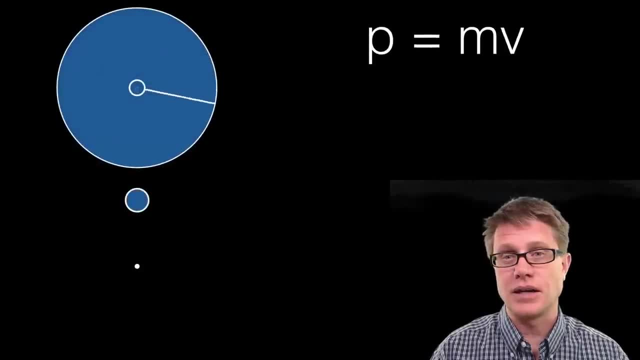 talking about angular momentum. So if we have a rotating disk like this, how do we calculate its angular momentum? Well, our equation is: L equals I times omega. In other words, the angular momentum equals the moment of inertia. So if we have a rotating disk like this, we 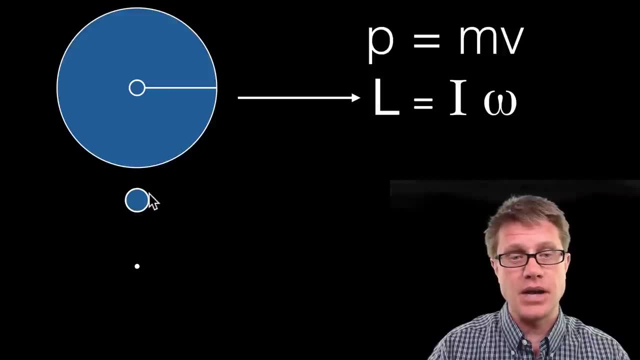 have moment of inertia, times the angular velocity. Let's say we have a point object like this in rotation, Then we are going to use a different equation. Now L equals RP, where R equals the radius, the distance from the center, And then this is going to be the linear momentum. 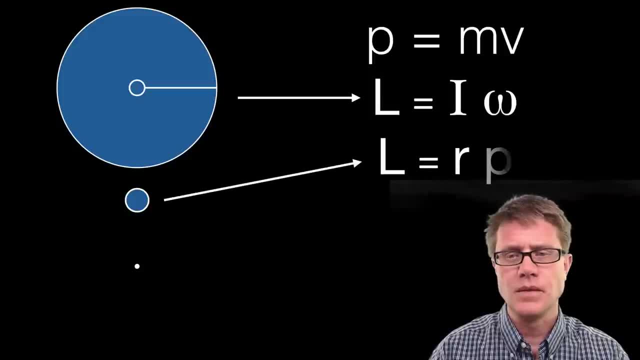 in rotation, Then we are going to use a different equation: Now L equals RP, where R equals the radius, the distance from the center, And then this is going to be the linear momentum. It is the linear momentum we were talking about just a second ago. So that is going. 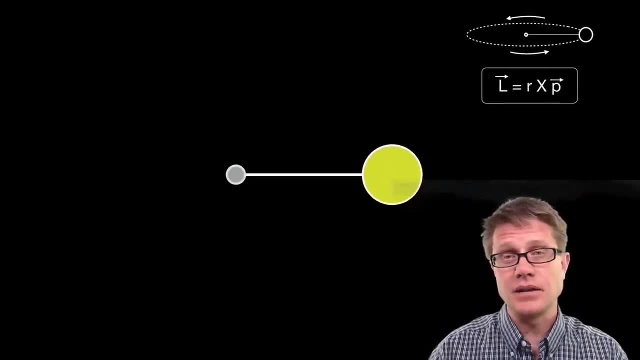 to be a product of the mass times, the velocity. Now let's look at this qualitatively. Let's say we have a tether ball, So it is a ball attached to a string And it is rotating around a pole like this, And then we were to quickly shorten up the radius. What would happen? 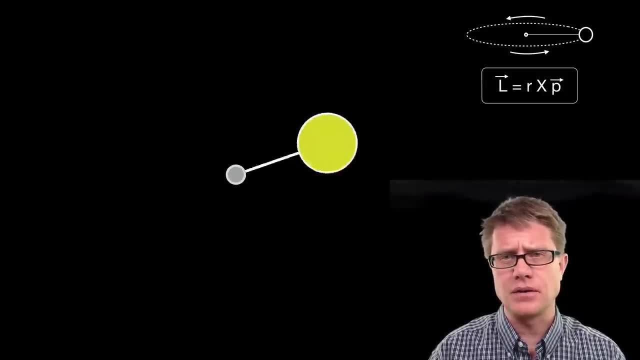 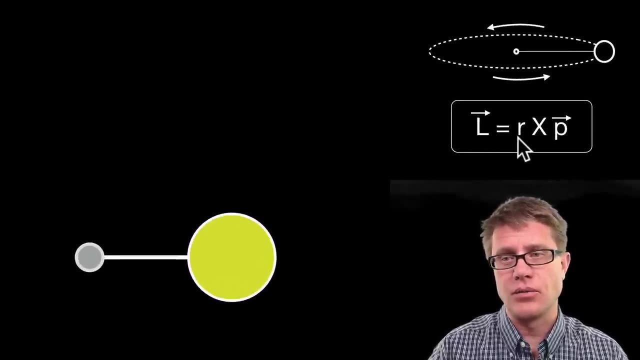 to the speed It is going to go much faster. Okay, Now that does kind of make sense. But why does that happen? Well, this was our angular momentum. before It was a product of the radius times, the linear momentum. Now we have decreased R, But our L is going to stay the same, So 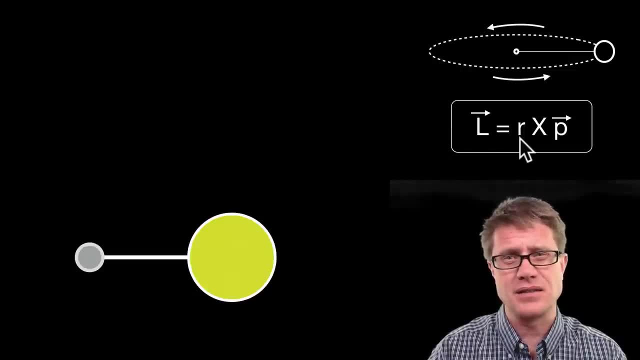 we are decreasing R. What do you think happens to the mass? The mass has to stay the same. And so what happens to the velocity? Well, the velocity is going to stay the same. So the velocity of the sphere, it is going to go up, So it is going to go way faster We 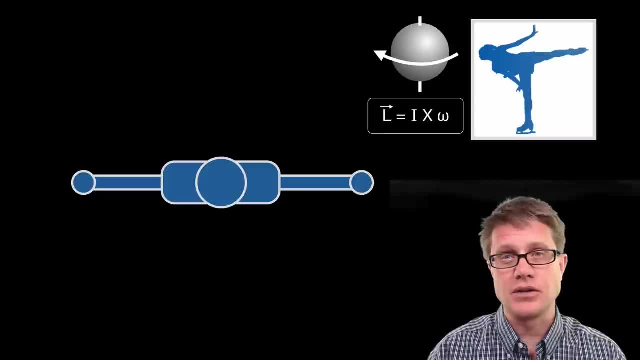 could apply the same thing to an extended object. Let's say we are looking at a figure skater and they are pulling their arms in. So let's say they are rotating, So it is an extended object, So they are rotating fairly slowly. And then what happens when they pull? 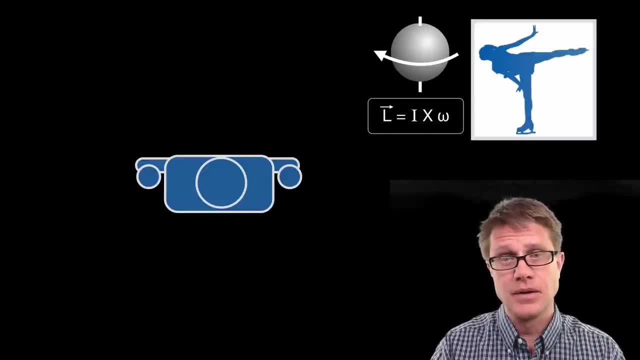 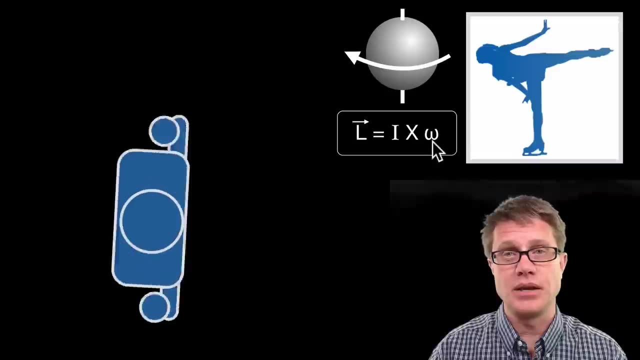 in their arms. Well, we are pulling more of that mass towards the center, And so what is happening? in this case? We are decreasing the moment of inertia. So what is going to happen to our angular velocity? It is going to speed up, And so the angular momentum. 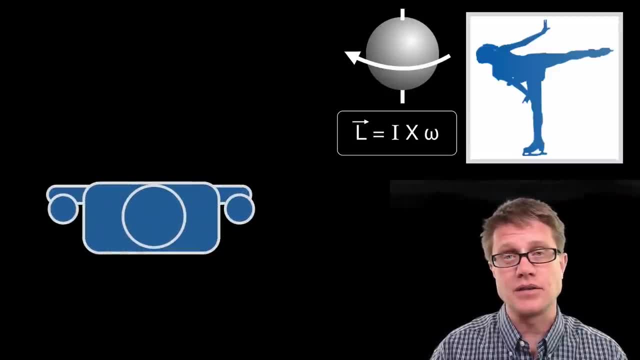 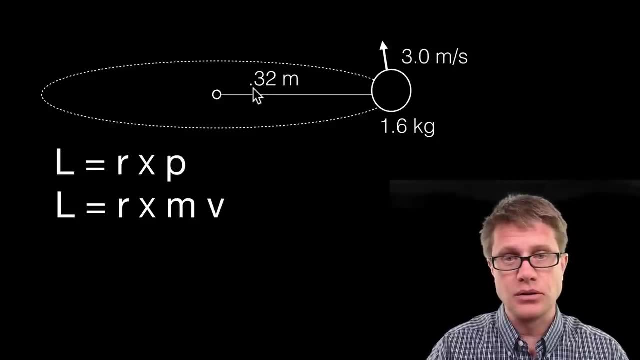 as conserved. it is just that we are increasing the angular velocity because we decreased that moment of inertia, And so we could do this quantitatively as well. Let's say we have an object, Now we will do a little bit of math. So this is the radius from the center. 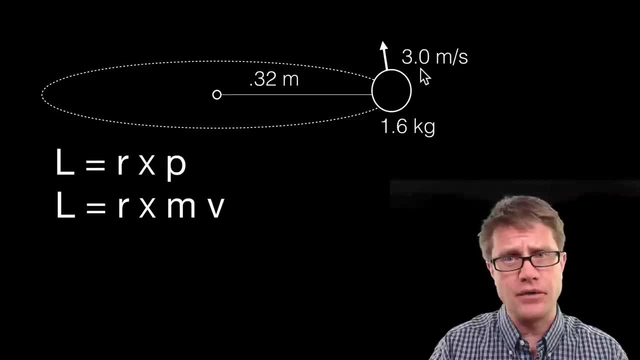 This is the linear velocity, how fast it is going in that direction, And then this is going to be the mass. And so, first of all, let's calculate the angular momentum before we change the system. And so I am going to plug in. here is my radius, Here is my mass. 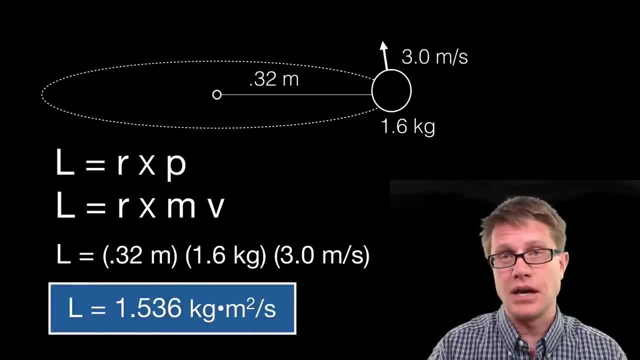 And then here is going to be my linear velocity, So I could calculate my angular momentum. And I am going to leave all the significant digits in it Because we are going to see what happens if we take the radius and we cut the radius in half. So we are going to 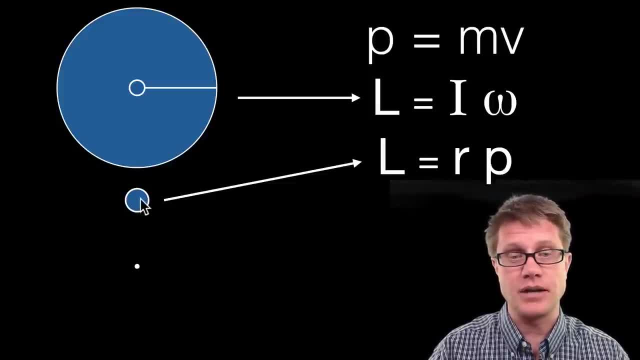 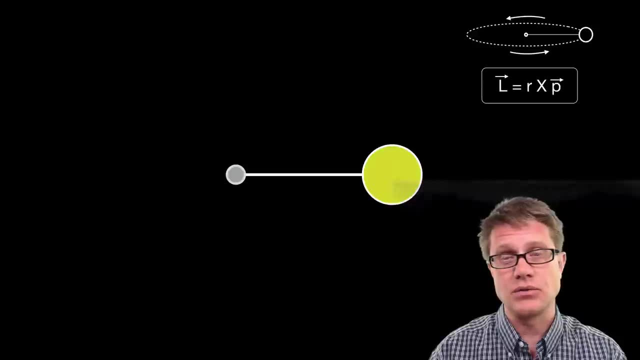 It is the linear momentum we were talking about just a second ago. So that is going to be a product of the mass times, the velocity. Now let's look at this qualitatively. Let's say we have a tether ball, So it is a ball attached to a string And it is rotating around. 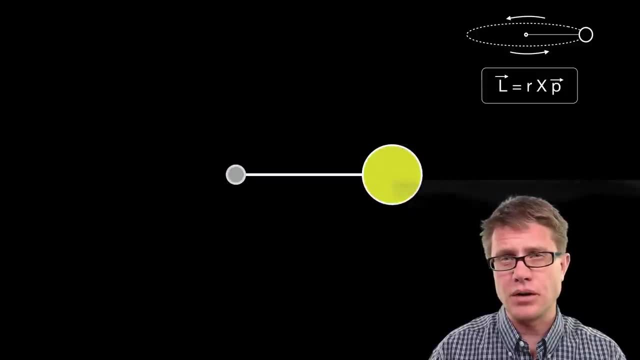 a pole like this, And then we were to quickly shorten up the radius. What would happen to the speed? It is going to go much faster. Okay, now that does kind of make sense. But why does that happen? Well, this was our angular momentum before. It was a product of the radius. 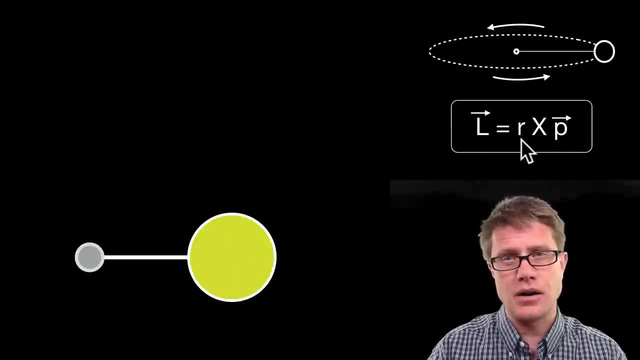 times the linear momentum. Now we have decreased R, but our L is going to stay the same, So we are decreasing R. What do you think happens to the mass? The mass has to stay the same, And so what happens to the velocity of the mass? Well, we have an angular momentum, So 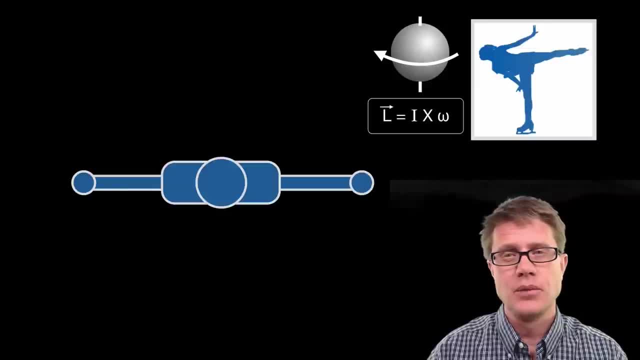 of the sphere. it is going to go up, So it is going to go way faster. We could apply the same thing to an extended object. Let's say we are looking at a figure skater and they are pulling their arms in. So let's say they are rotating, So it is an extended object. 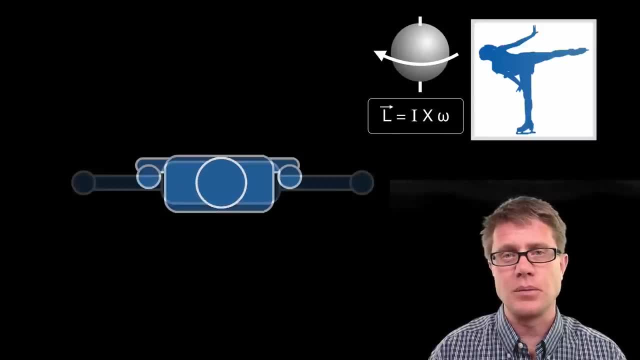 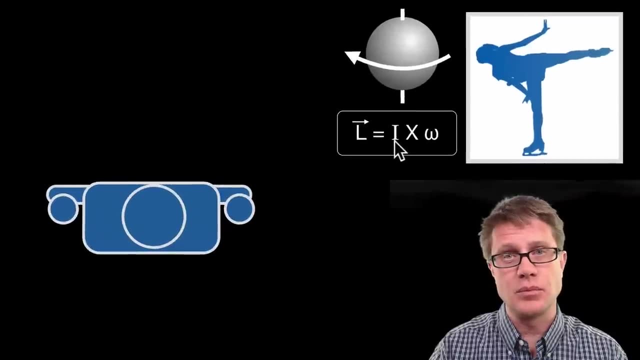 So they are rotating fairly slowly. And then what happens when they pull in their arms? Well, we are pulling more of that mass towards the center. And so what is happening? in this case, We are decreasing the moment of inertia. So what is going to happen to our angular 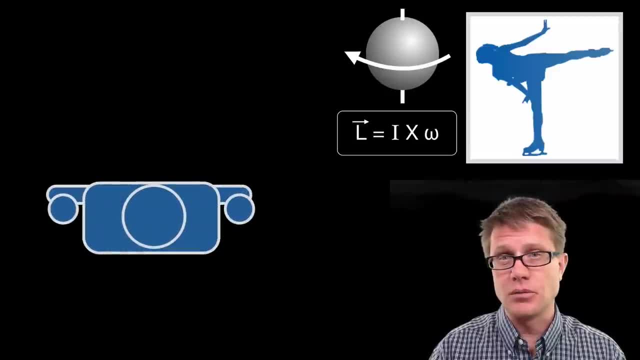 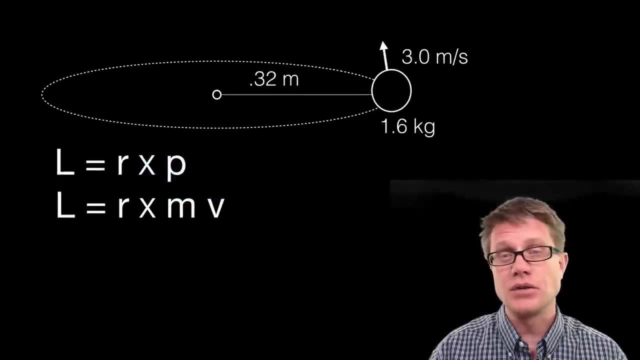 velocity. It is going to speed up, And so the angular momentum is conserved. It is just that we are increasing the angular velocity because we decreased that moment of inertia, And so we could do this quantitatively as well. Let's say we have an object, Now we 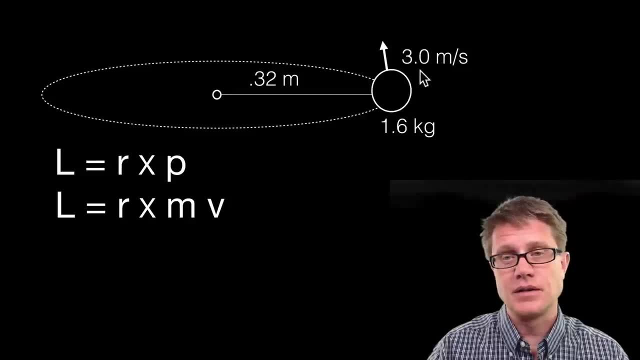 will do a little bit of math. So this is the radius from the center, This is the linear velocity, how fast it is going in that direction, And then this is going to be the mass. And so first of all, let's calculate the angular momentum before we change the system. And 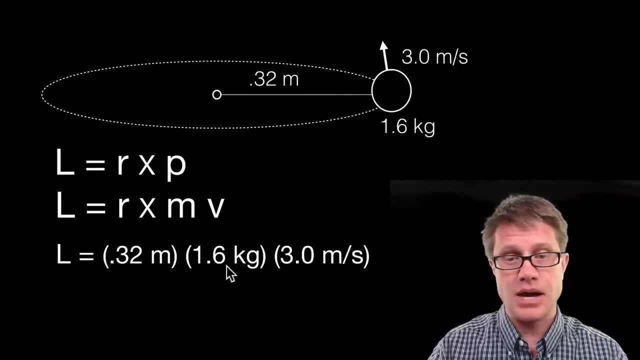 so I am going to plug in: here is my radius, Here is my mass, And then here is going to be my linear velocity, So I could calculate my angular momentum. And I am going to leave all the significant digits in it, Because we are going to see what happens if we take 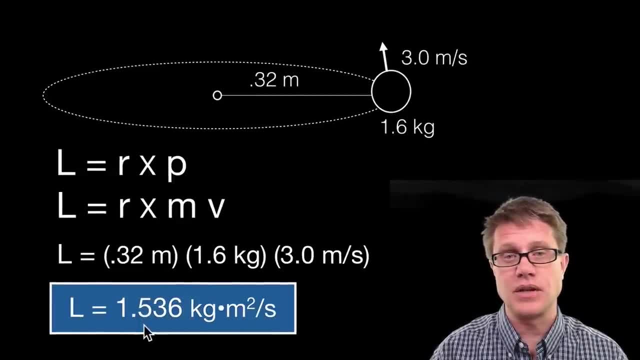 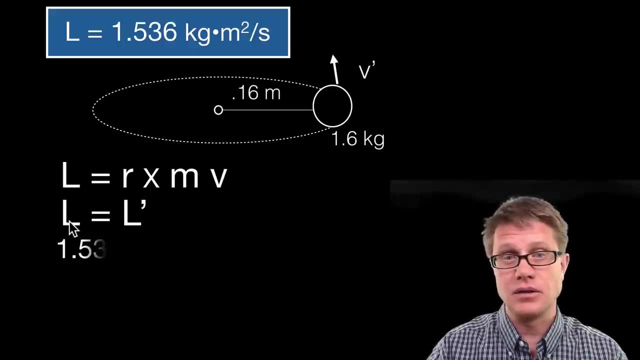 the radius and we cut the radius in half, So we are going to decrease that radius, So now it is 0.16 meters. And so I know this. I know my initial angular momentum And now we are going to solve for my angular momentum after we have reduced that moment of inertia.